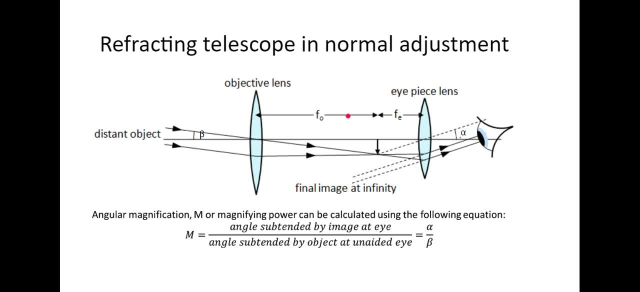 the objective lens, so O for objective lens. So that's that first the left hand side of the diagram. Now, if we switch to the second diagram, that second part of the diagram, so we just look at the right hand side now and again. just, 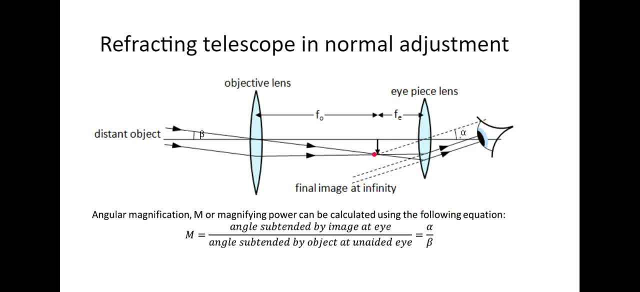 ignore the left hand side for a minute. So here now, what was the image is now the object for us. so here, if we draw a ray going through horizontally and then it goes through the focal point over here, and then this ray here, or it's actually 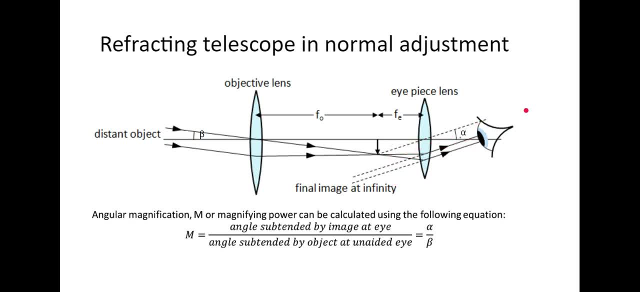 this ray over here, but they're parallel- is just going in a straight line. Okay, so these two rays end up traveling parallel to each other, and so this is what I was saying earlier: that the image will be over here. so you trace the rays. 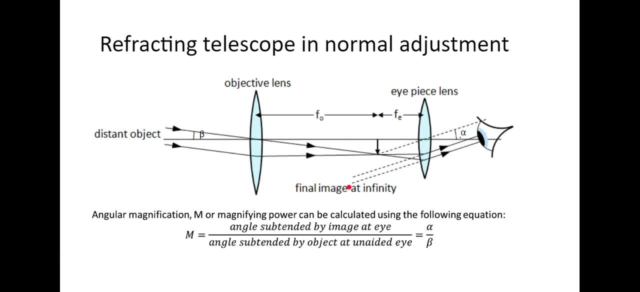 back and the image will be at infinity, and so, therefore, when you're looking through the telescope, your eyes are focusing on infinity, just like they would be if you were looking at the stars in the sky. Okay, so hopefully that makes the diagram not quite as complicated. 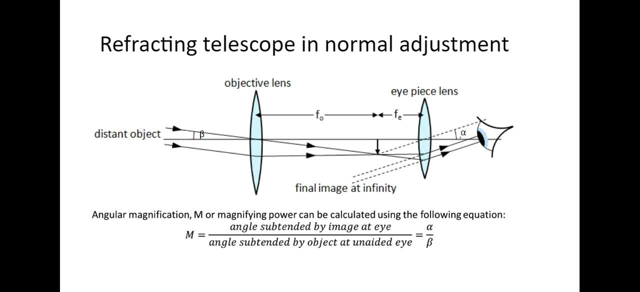 As it did, as it seemed before. I asked you to copy down this diagram before the lesson, if possible. if not, just make sure you've got it, because they quite often ask this in exams: to draw a ray diagram for a refracting telescope in. 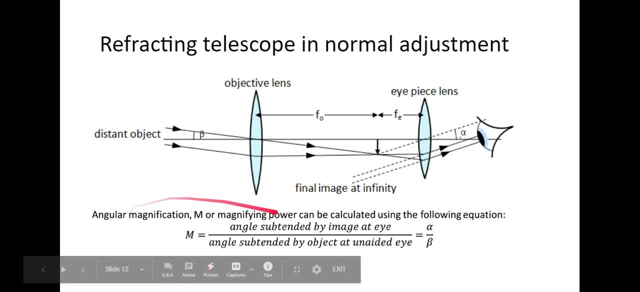 normal adjustment. that's just what this is called. An important thing to note is that the length of the telescope is determined by the two lenses, because the scope has to be the focal lengths of the two lenses added together and because that gives us this special case where the image of the objective lens is then. 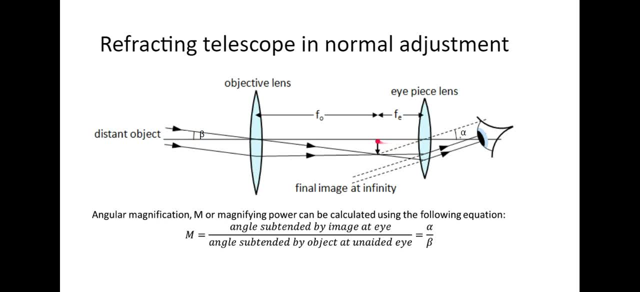 at the focal point of the eyepiece lens. Okay, so the length is always going to be fo plus fe, so it's an important thing to note down. And also, you need to think about these two angles. okay so these two angles determine how magnified the object is. okay, so that's why we use. 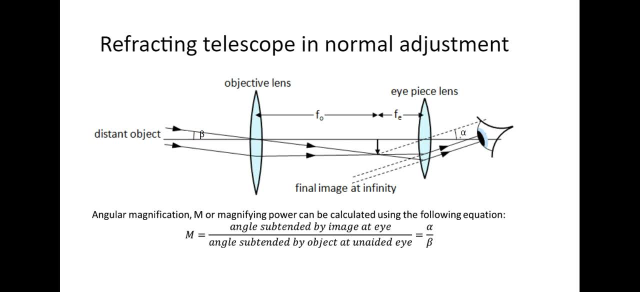 telescopes. isn't it to magnify things so that you can see them more clearly? and if you just look at those two angles, you can see that alpha is bigger than beta and the ratio of how big they are compared to each other determines how magnified it is. 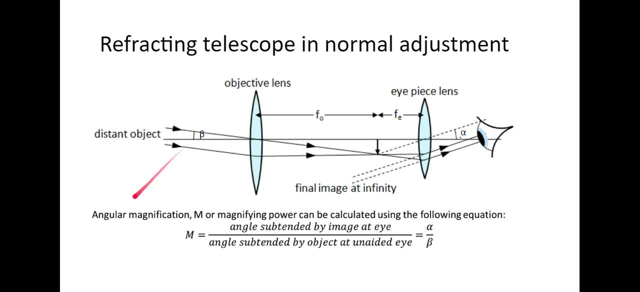 which hopefully that makes sense. and now in your data booklet you're given this equation but you're not given alpha over beta or you're not told what alpha and beta are. okay, so you've got to understand or remember what these mean, and they've got waffly fancy words and so it can sometimes be a bit confusing. 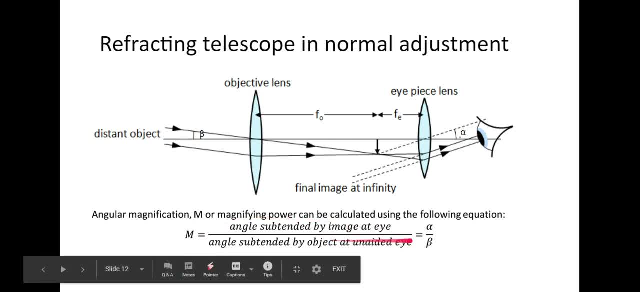 when you see in your data booklet this bit: m equals angle subtended by image at divided by angle subtended by object at unaided i. it is all just a bit flowery and so it's hard to remember what that actually means. so angle. 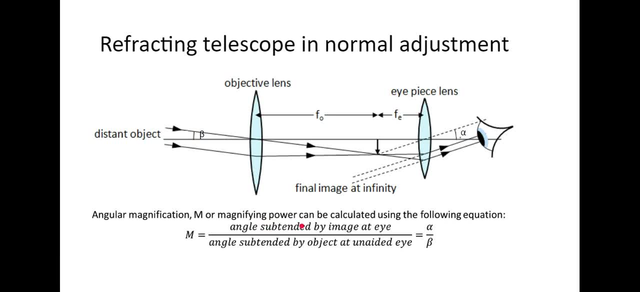 subtended just means angle made by. okay, so I I think it's the angle made by the image at the eye. so that means you're at the image at the eye. so that means it's a bucket of data for you to use, right, right. 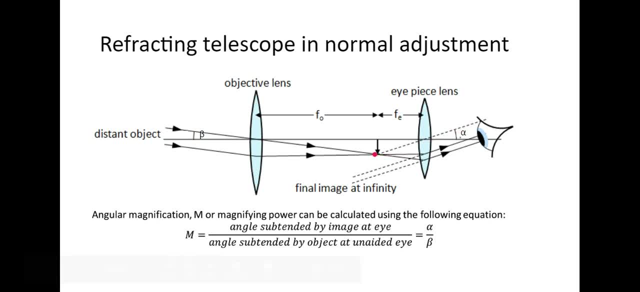 eye, so it's this angle here. so this is the image, so it's this angle, alpha, okay, so this one is the one closest to your eye. so you can think of it like alpha is the first in the alphabet, so it's the one closest to the eye. that's one way of remembering the other angle angle subtended by. 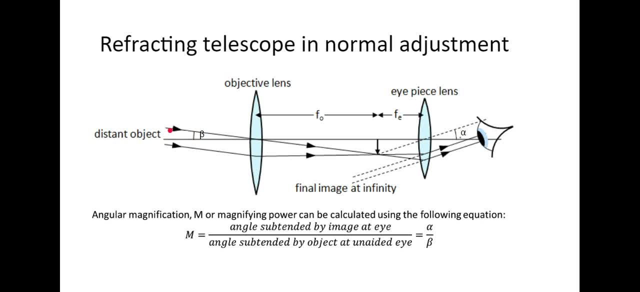 the objects. there's a object at the unaided I, so RI is basically on this principal axis and says the angle between those two. okay, so the magnification is the ratio of those two angles. okay, and you are given that in the data but click and the other equation that you give them. 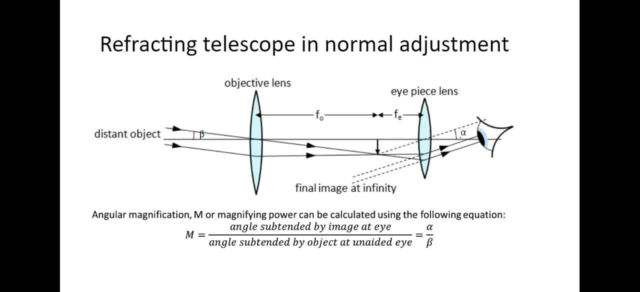 and I'm going to show you how we get to that. the other equation you don't need to know how you get two of. it is quite straightforward. So for this one, we need to think about this bit here. So we have a height of this image, which is y, and that creates two triangles. So we've got one triangle. 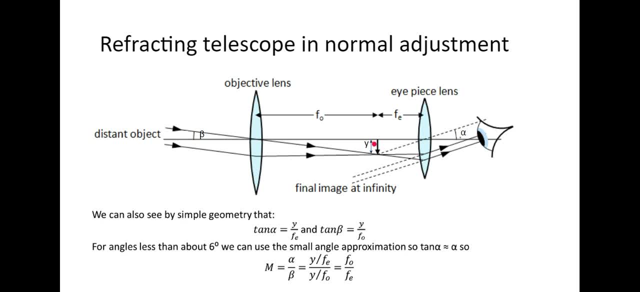 on this side and then we've got a smaller triangle to the right of that arrow. And we also know the lengths here, because these are the focal lengths. So this is fe and then this bit is fo. We also know the angles because the angle here. so this angle over on this. 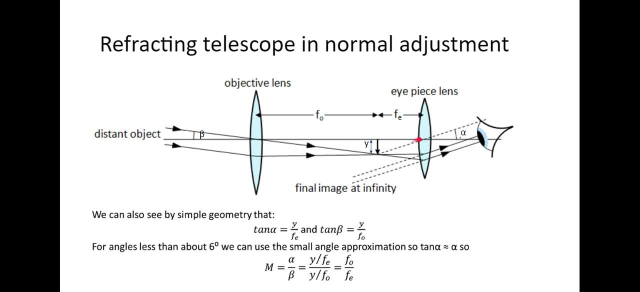 side is alpha. so that's geometry, because they're z angles and this angle here would therefore be beta. So we know one of the lengths of the size and we know one of the angles. so that means we can use trigonometry to work out what y is. 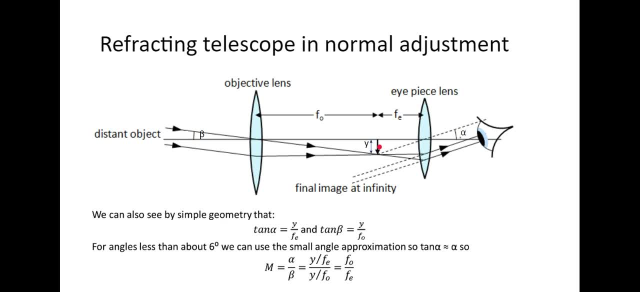 And y is obviously the same for both of them, so that makes life easy as well. So we've got y, we've got fo and fe. So if we look at this triangle, first of all we've got y and fe. we don't know what the hypotenuse is. 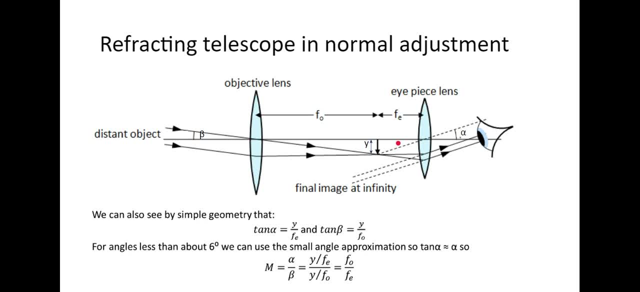 but we know this angle. so if we know the angle, we know the opposite and we know the adjacent, then we know that the tan of the angle, so tan alpha, is opposite y over fe. okay, so tan alpha equals y over fe, and then, likewise, for this side, tan of beta would be y over fo. okay, so that's this. 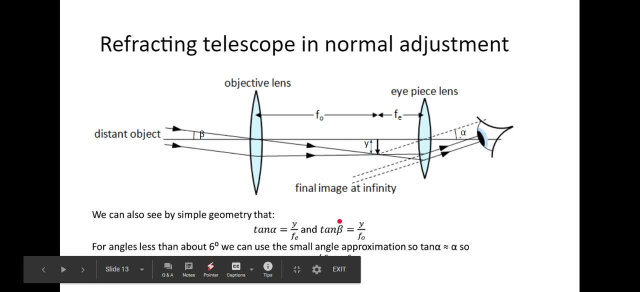 little equation here, but we also know that, um, these angles are going to be very small, okay, because most of the things that we're looking at are very straight up, so the angles are tiny. um, so we can use what's called the small angle approximation, which we i talked about when we 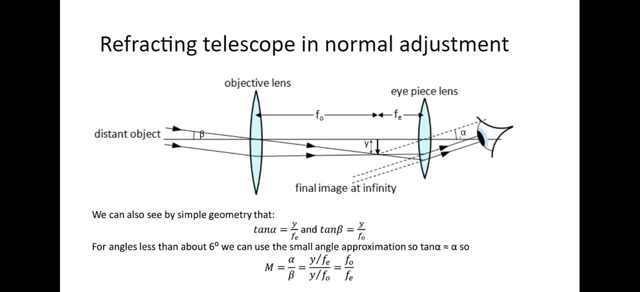 were doing diffraction gratings, and that just means that tan alpha is approximately equal to alpha. so therefore we can get rid of that tan bit, because that confuses things um. so um, i've got to stop moving my cursor so you can see it. so n we know from previous slide. 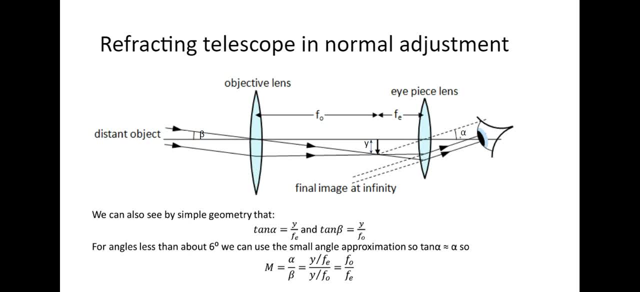 is alpha over beta, the ratio of those two angles. but we also know tan alpha is y over fe. so therefore, because of small angle approximation, alpha equals y over fe and beta equals y over fo. so therefore we can just substitute that in so alpha is y over fe. 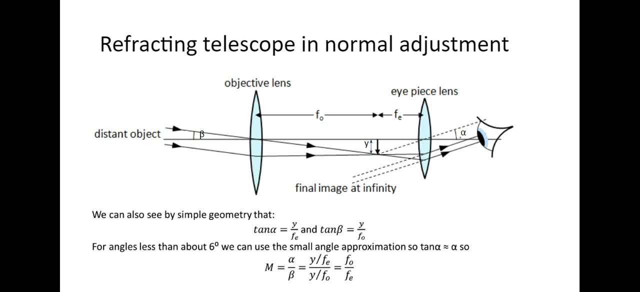 beta, y over fo, and because the y's are the same, they cancel. so you've got one over fe, divided by one over fo, which basically flips up the other way, and you get fo over fe. okay, and this is a much more useful equation because, um, the angles are quite difficult to. 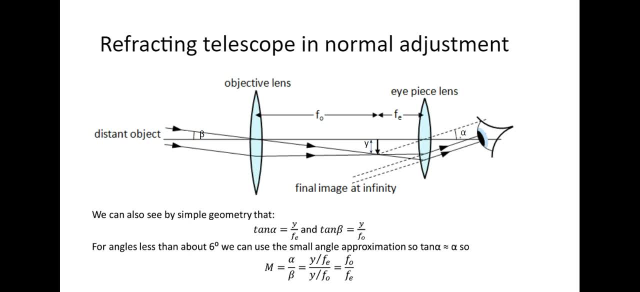 measure. but the focal lengths are very easy to measure because you, when you've made or bought the lenses, you know what focal length you can measure and you can measure focal length. you can measure that focal length, you can measure that focal length. you can measure that focal length you can measure. 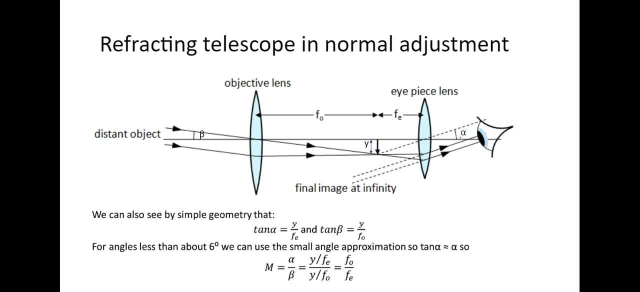 easy if you don't know what they are. you can easily measure the focal length of lenses when you buy a telescope. you're going to know what they are because it'll tell you, and so that's a much more useful equation. so fo over fe, okay, and again that m equals fo over fe is given to you in the. 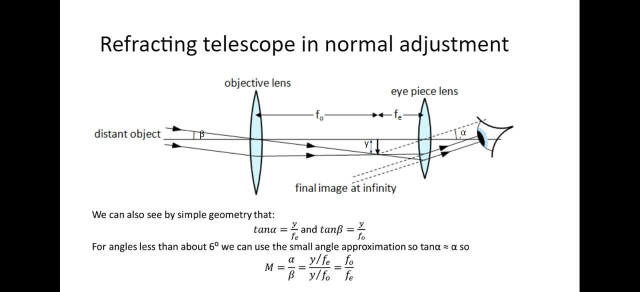 data booklet. um, not all the rest of it, but you don't, you wouldn't need to know how to get from one to the other. okay, so that is how a refracting telescope works. okay, so it takes, takes light in from the objective lens, focuses at a point and then the eyepiece lens, then, um, uh, takes the light. 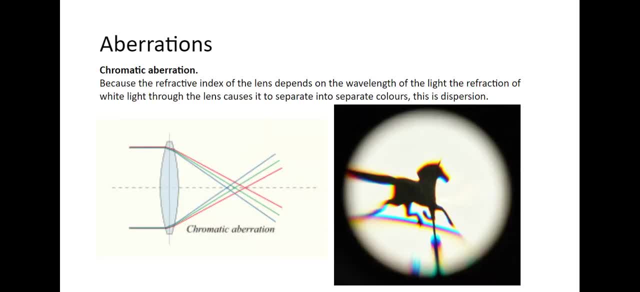 and sends it to your eye. hey, um, just need to talk to you. um, through a few problems with lenses, um, and these are called aberrations, which is a posh way of saying problems, um. so this first one is called the chromatic aberration and a chromatic aberration is um, so aberration means problem, chromatic color, okay, so it is to. 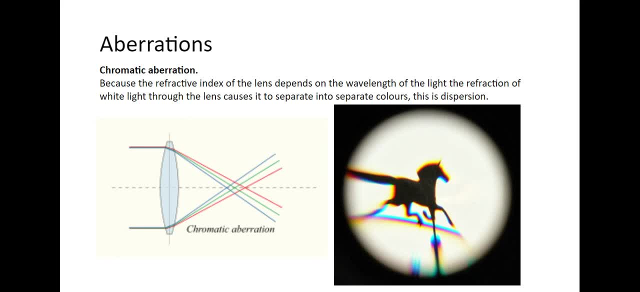 do with wavelengths, and this is because, as hopefully you remember from the waves topic, the lens refracts the light but it has the refractive index of the lens um changes depending on the wavelength. so different wavelengths have different refractive indices of the lens, so they are refracted by different amounts. okay, so each of the colors there you can. 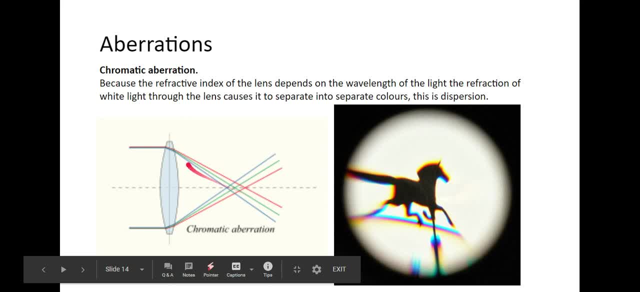 see are refracted by different amounts on here, and so it ends up with this blurring. they're not all focused in at the same point. so here's an image of a weather vane. so you've got the horse. so you've got the main bit, is fine. but around the edge of the vane you've got the light and the 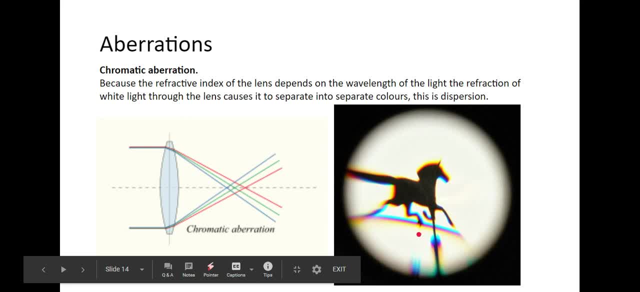 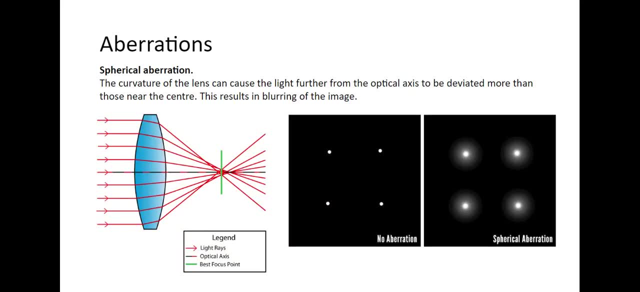 you've got a blurring of this- uh, rainbow colors- where it's just spreading out. okay, so you've got that dispersion effect. and the other type of aberration you need to know about is called spherical aberration, um, and this is due to the curvature of the lens, so i said this had to be. 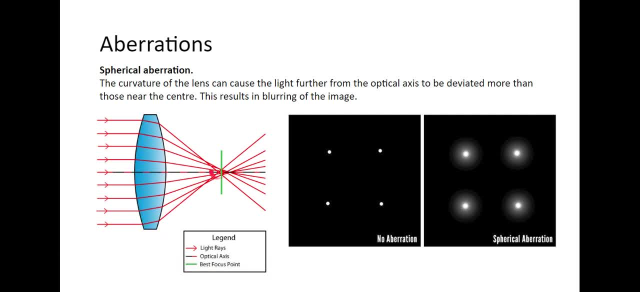 very precise in order to get all the rays focused at the right point. um, so if that's not done quite right, uh, so maybe cheaper lenses or not quite right? uh. so if that's not done quite right, uh, so maybe cheaper lenses or not quite right? uh, so, maybe cheaper lenses, or not quite right? uh, so maybe. 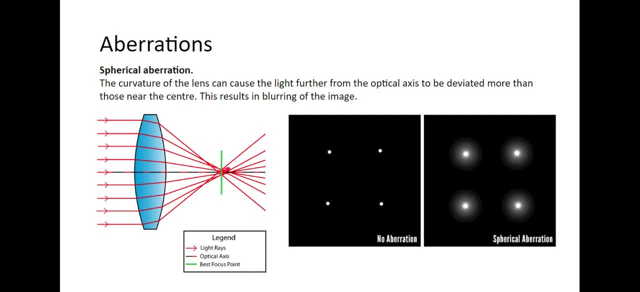 cheaper lenses or not quite so well made, then they don't all meet at the same point. okay, um, so this is what you should get if there was no aberration. so you get nice, four nice circles of bright light. but if there is aberration, if there is this spherical aberration, you get. 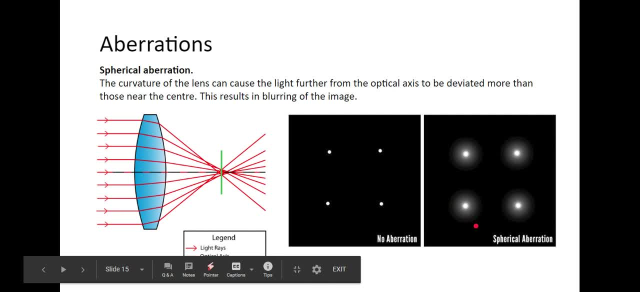 a blurring around the edge. okay, so it's all fuzzy. so if you're looking at a star or a planet through, um, your telescope or whatever it's going to be in terms of color, it looked about this, or I thought of burning prices and it wasn't done properly. you know the ignor可能现那儿. 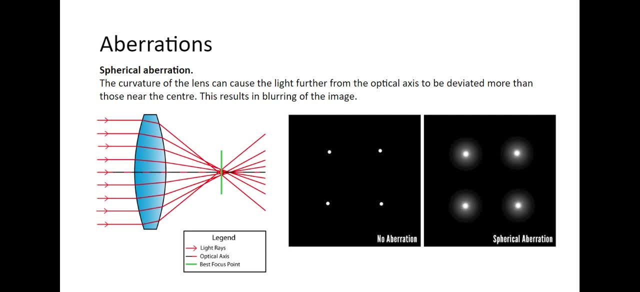 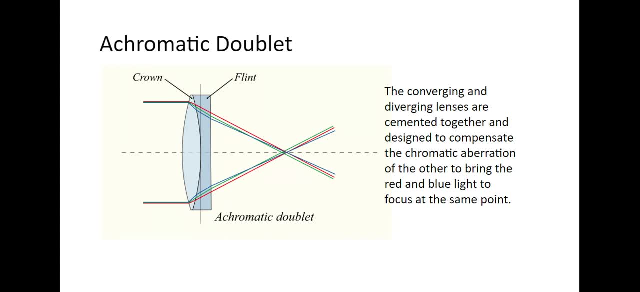 a test flavor and smother. there was one kind of sort of pigeon coverin' positively surrounding the to look a bit blurry so you don't get a nice clear shot of the image. So how can you fix this? So this is how we can fix the chromatic aberration and it's called an achromatic doublet. Doublet because